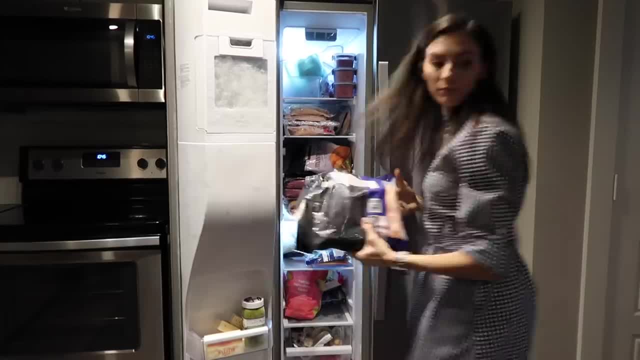 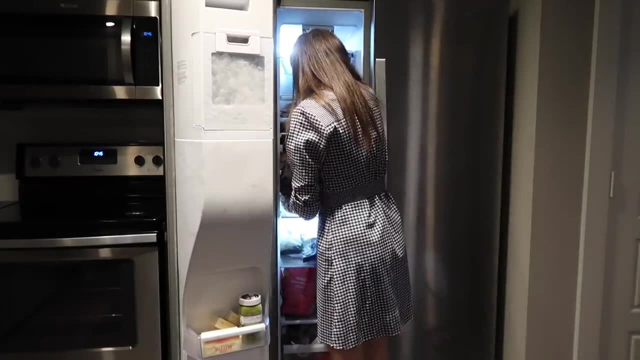 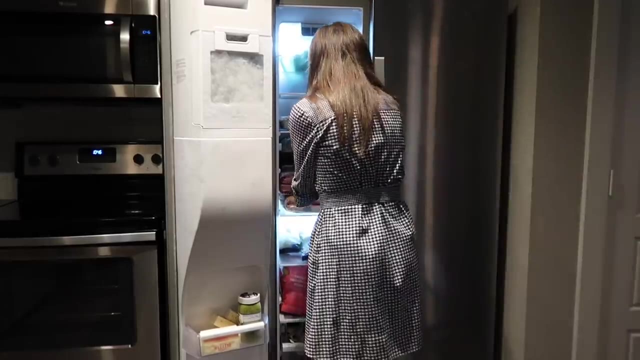 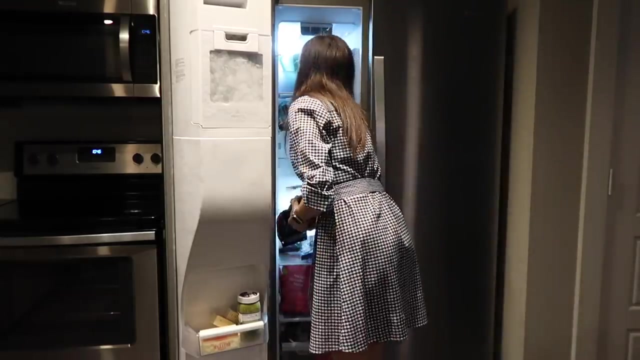 ground beef, all of that. The prices at Costco are pretty good and we both like eating meat, so I just stock up every single time I go to Costco so I don't have to go there as often. But I will say this is the most meat I will have in the freezer at any given time. This is. 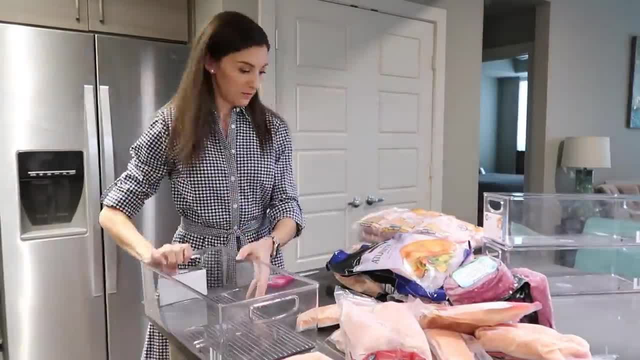 completely stocked up and potentially slightly overstocked up. for us, especially when you look at it all on the countertop like that, That looks like a ton. So I'm going to start with the meat. I'm going to start with the meat I'm going to start with. 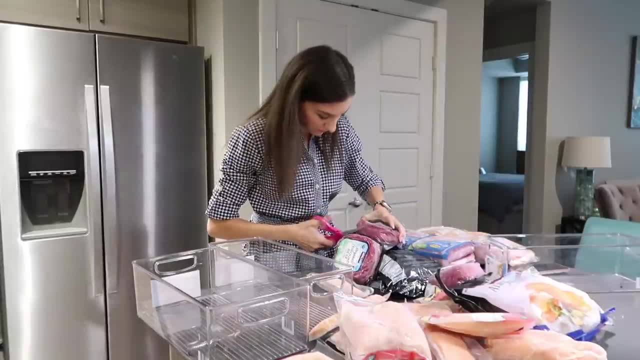 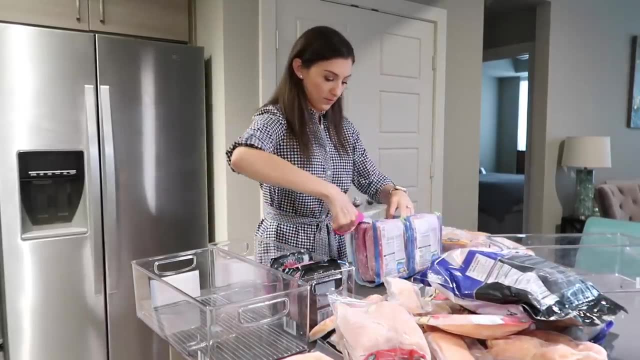 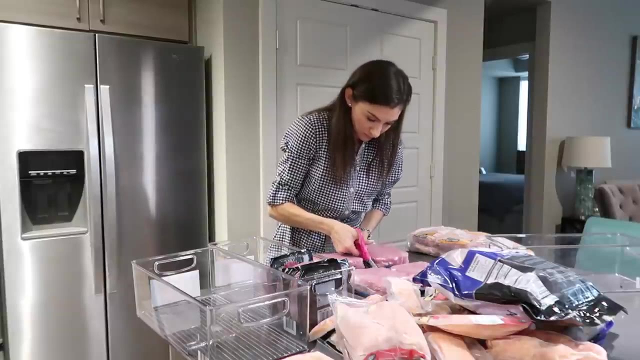 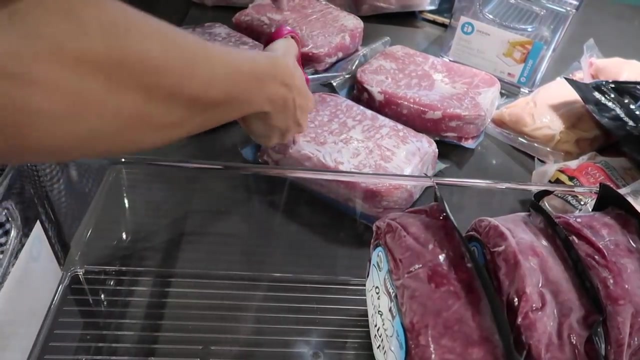 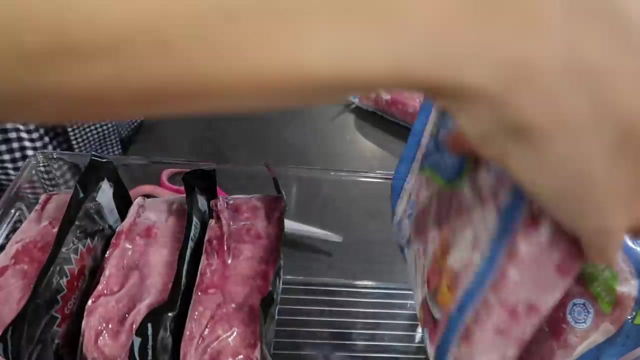 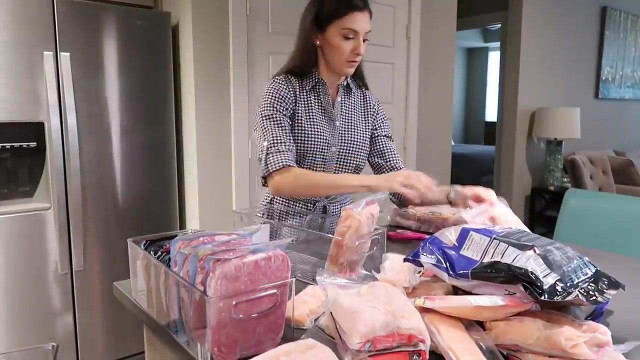 the meat. I ordered three bins from the container store and I will link them in the description box below. but I wanted to try and kind of play around with which things worked best in them and figure out how to best organize the products. I got to find the way. before it disappears, I cannot stay. 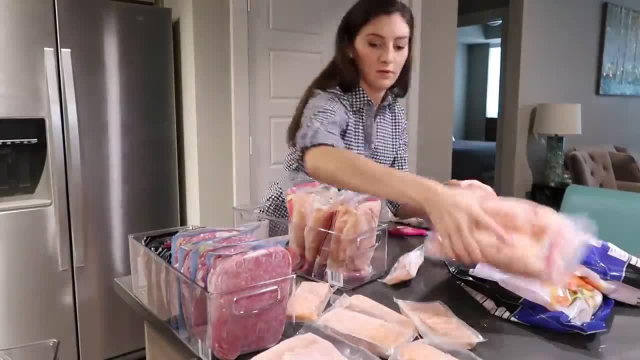 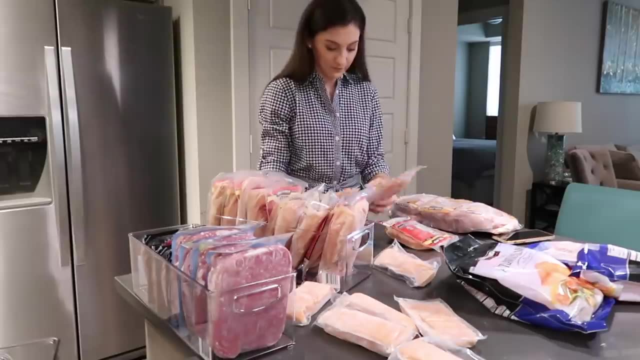 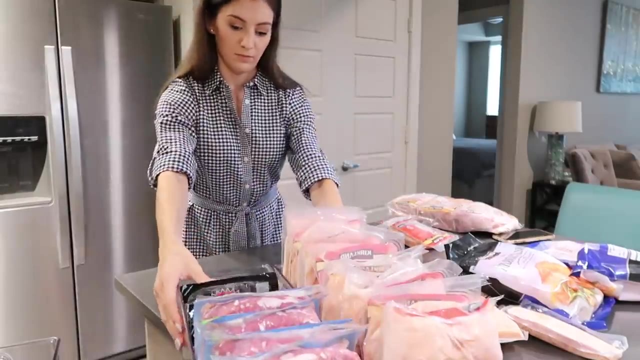 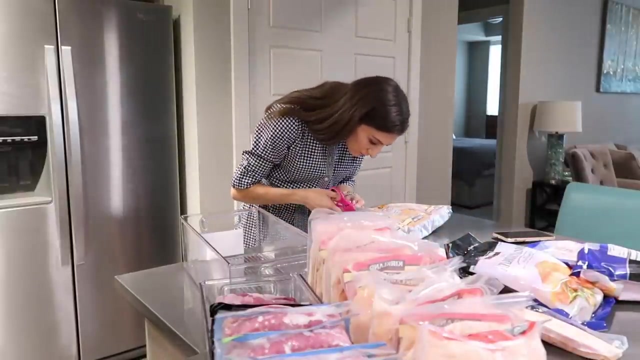 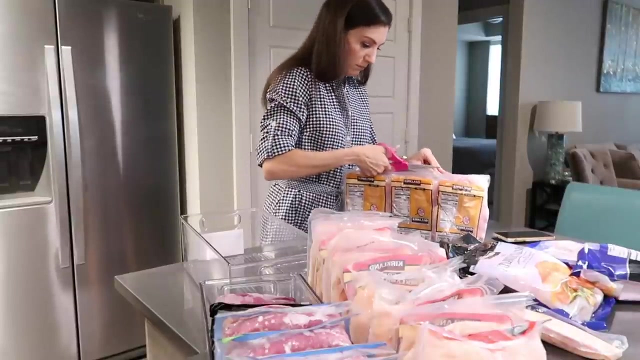 I feel the pressure on me, How it's itching under my own skin. It's getting real hard to breathe. I got to move on. Got to move on right now, Yeah, so this is really frustrating because i always try and separate and cut apart all of my chicken. 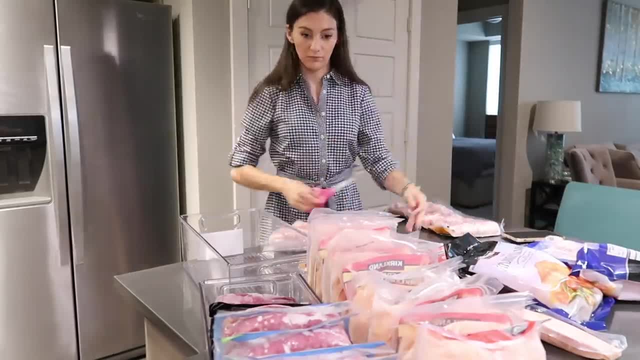 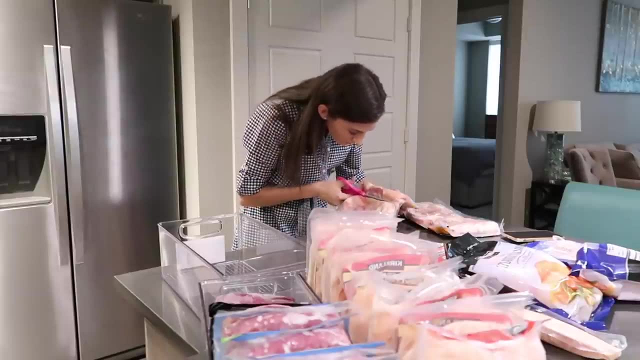 breasts and meat products from costco before i freeze them. just because the margin of error is so small between the two packages and if you freeze it first and then try and cut it later, sometimes the way it freezes, it's really hard to get the scissors in between. 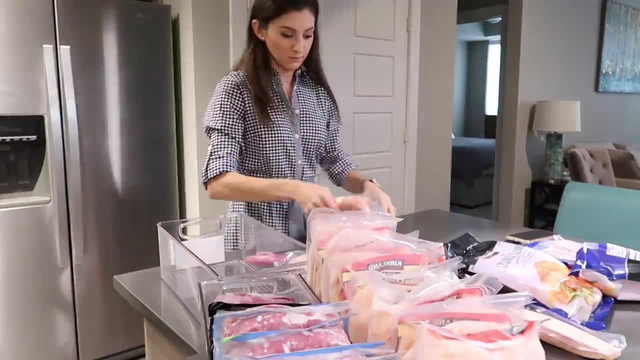 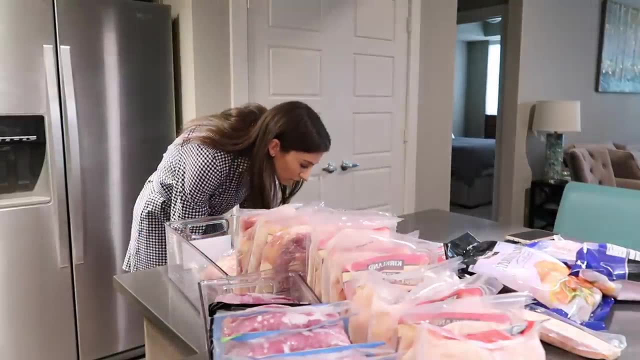 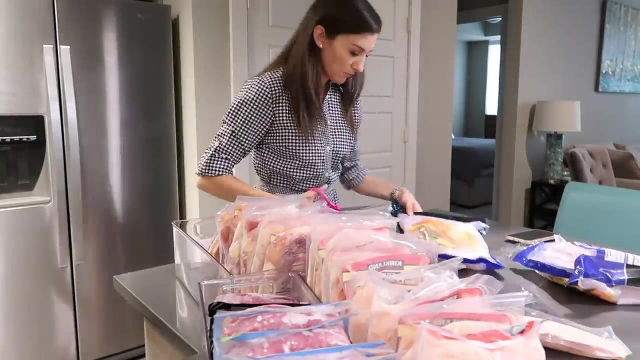 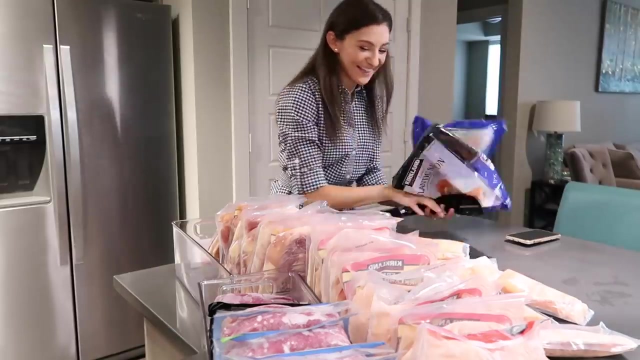 so i would definitely recommend cutting, then freezing. if you haven't tried the frozen salmon from costco, i would definitely recommend it. it's one of our favorites. we both really like salmon and it's something i really like about the frozen salmon: it's really easy to cut and it's really easy to. 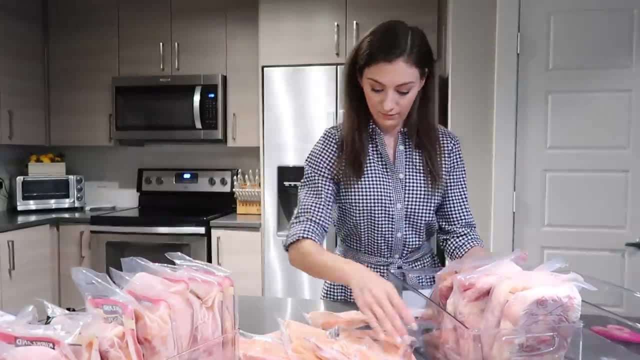 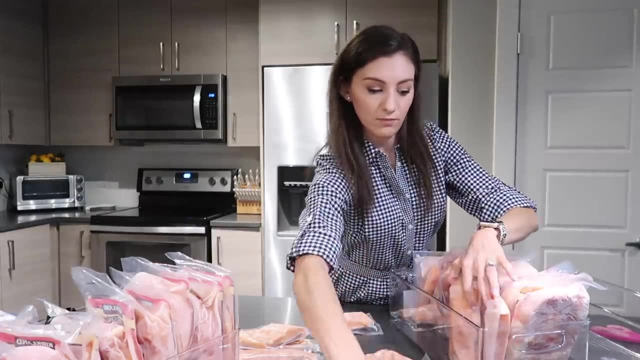 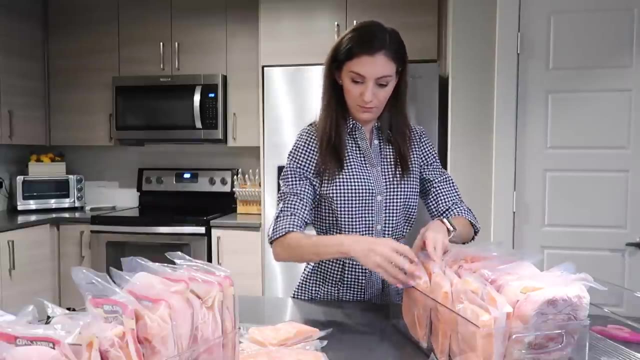 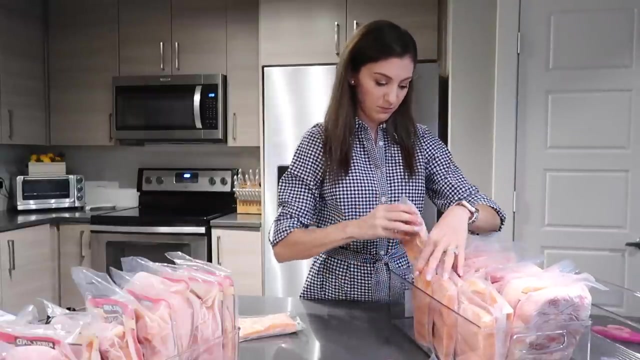 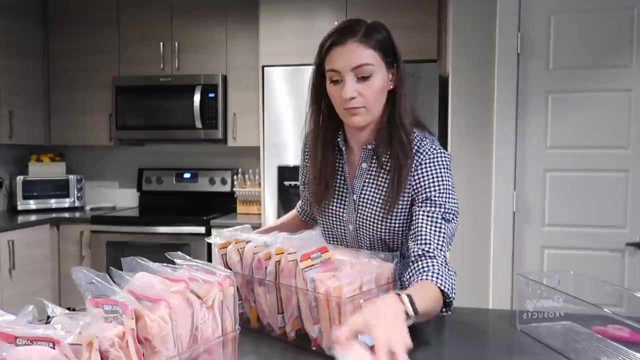 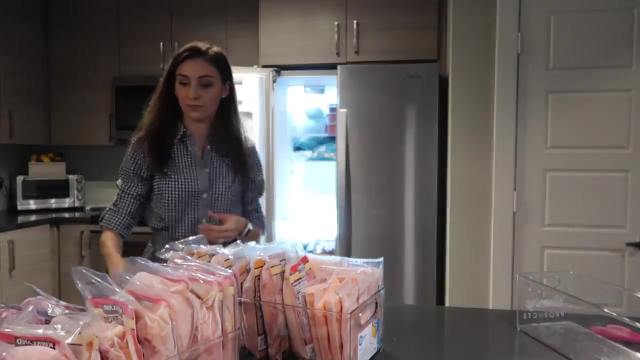 i would honestly probably even serve at a dinner party. you can't really tell that it's frozen salmon and it's great. lately nothing goes in my direction. lately nothing's coming my way. keep drowning everybody. a difficult part always of fridge and freezer organization is working as quickly and efficiently. 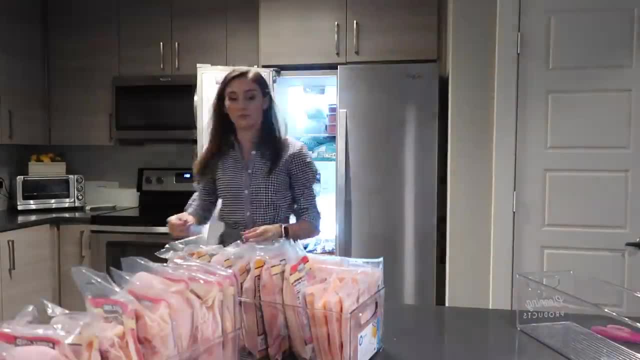 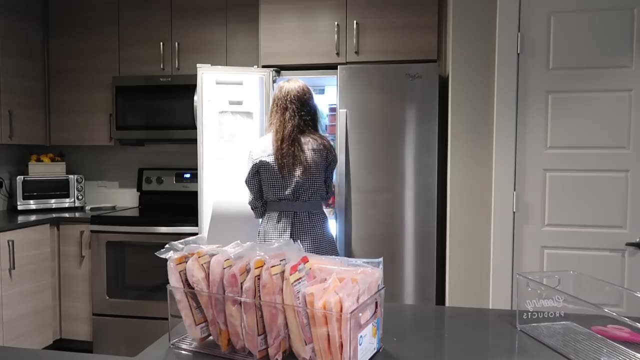 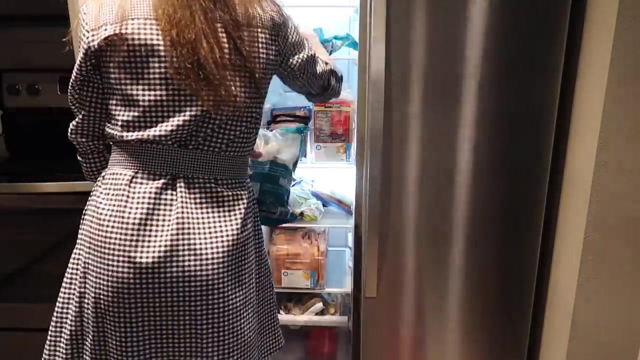 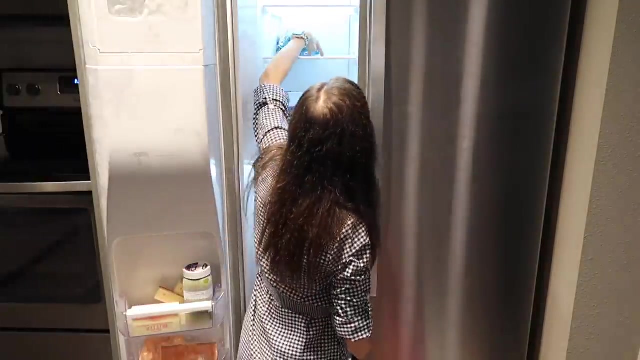 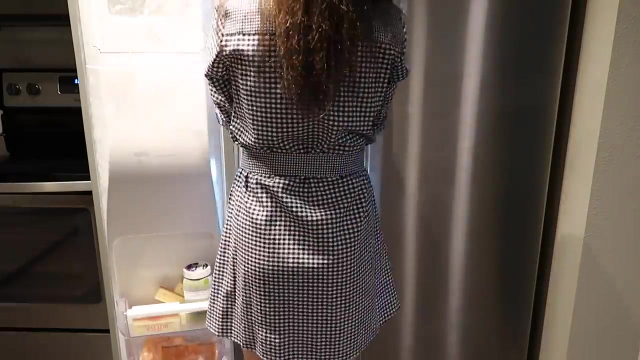 as you can, because you definitely don't want to keep those doors open for too long, because you don't want your food being exposed to the regular air temperature, but also, of course, you want to save as much energy and electricity as you can and to realize. so you'll see, with my smoothies i did have them in a little bit of a shorter container and i wanted 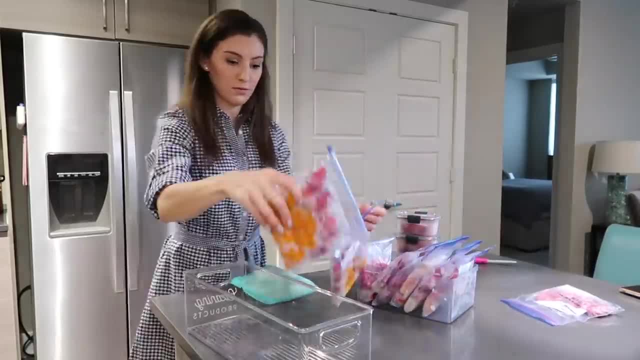 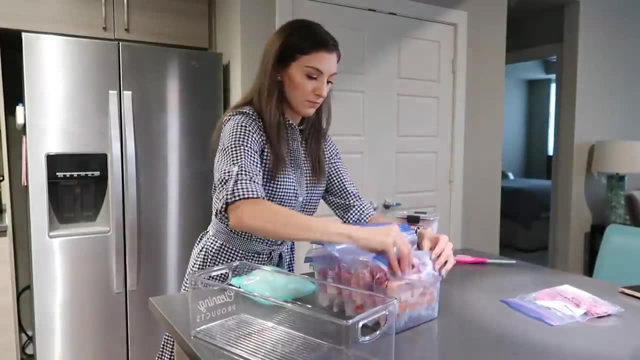 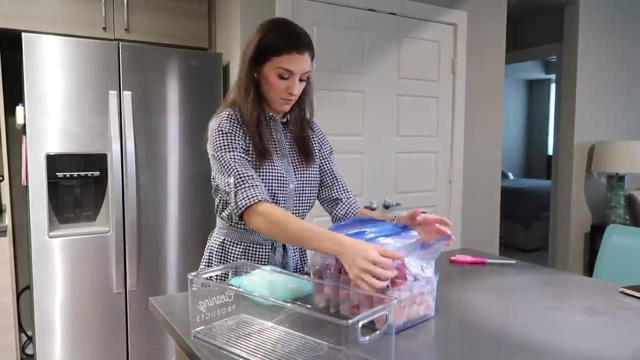 to play around with whether they fit better in one of the old containers, but this short container was the only bin that i had in my last freezer, so this concept of using bins to organize my freezer is definitely new to me, but this short one actually works really well in a 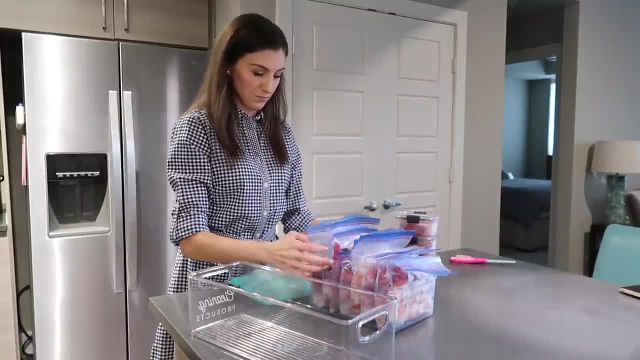 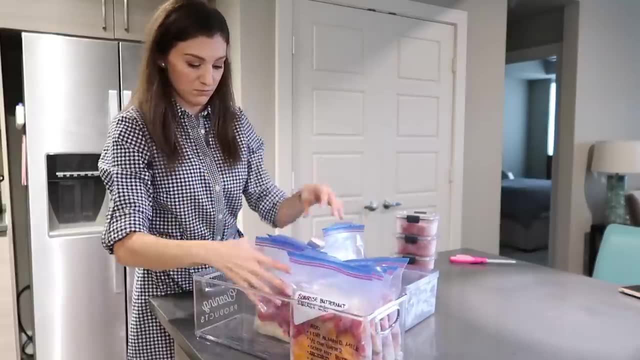 spot in the freezer that has a light behind it, where i can't fit the long bins like they fit on every other shelf, and i do like to do some pre-packaged smoothies. especially there's this one smoothie that i really like that i will be sharing with you guys in my upcoming smoothie. 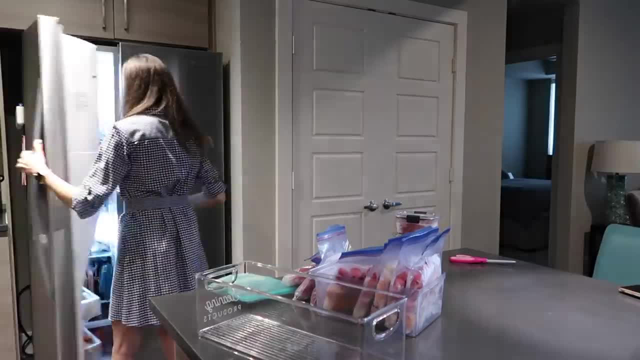 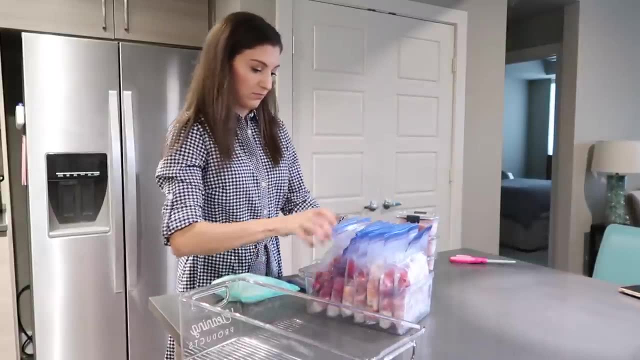 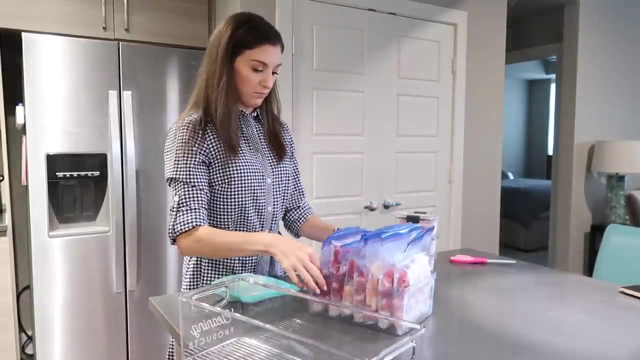 video. but it has butternut squash in it and that is a pain in the rear to measure when it's already frozen. so i measure it when i cook it and then freeze it right away in those freezer bags, and i do hope to get more stasher bags or reusable silicone ziploc type bags so i don't have to be. 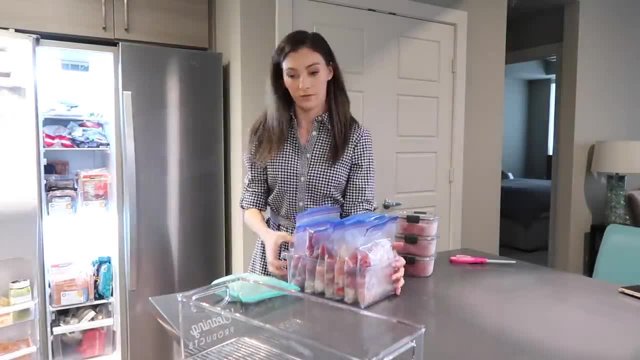 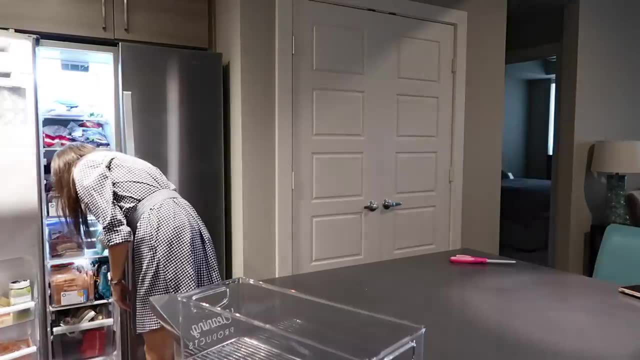 so wasteful with ziploc baggies, but i don't have them yet. i'm hoping to get them at some point. but i will link the stasher bag in the description box below because the one that i have i always use for frozen bananas and love it. you can stick it in the dishwasher, it's great. 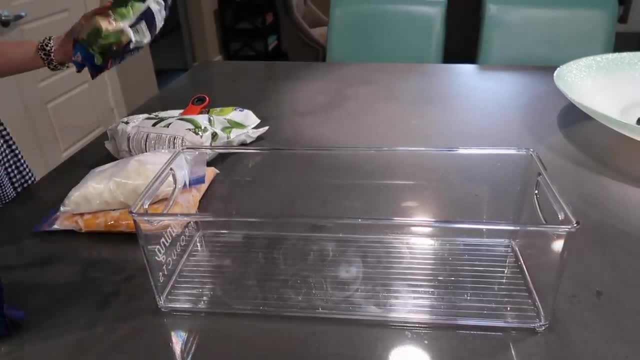 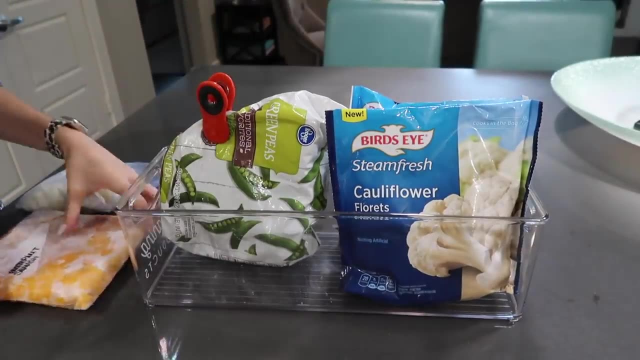 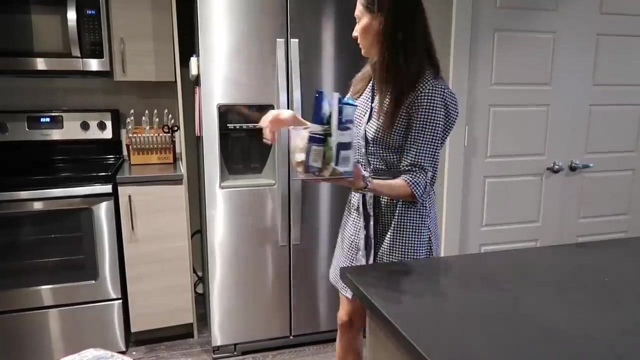 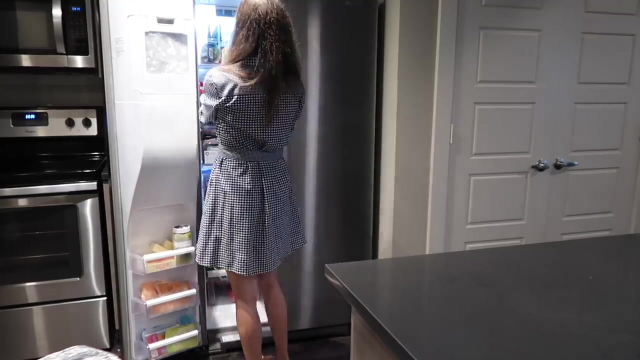 so i don't have a ton of frozen veggies, but i do want a separate container just for frozen veggies, because i do always have something on hand and it will leave me a little bit of room to grow. so i do have a lot of frozen fruit and i have always loved putting the frozen fruit. 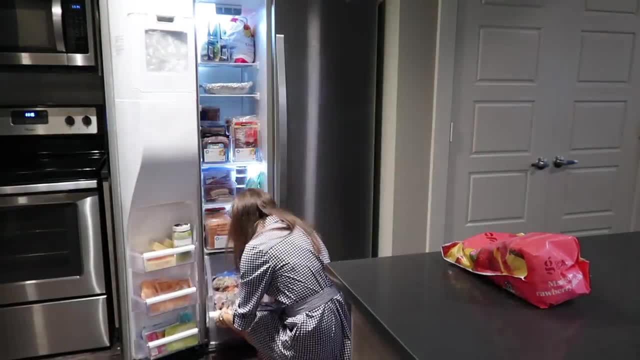 because it's just really filling up my fridge and my alsap or your freezer making onions, but because they come in such large bags at the bottom of the freezer in that pull-out drawer. So that's what I'm going to do right now and fill it up with all my fruit. 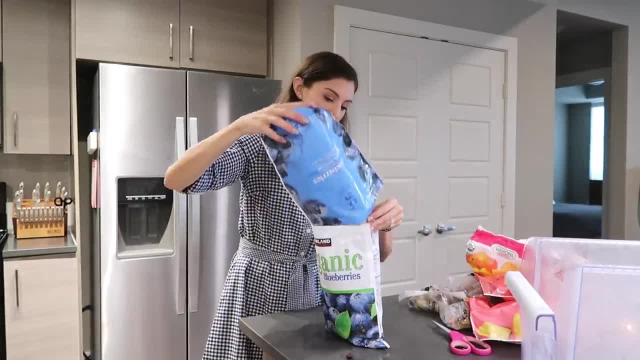 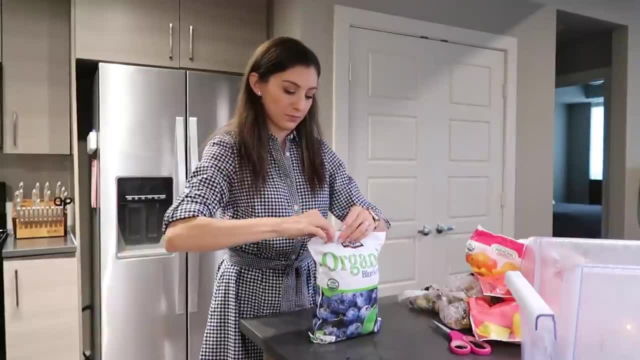 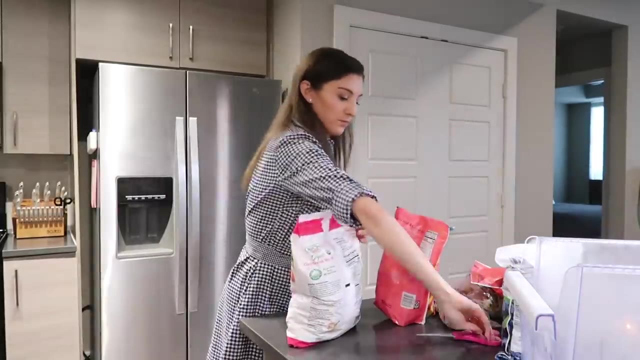 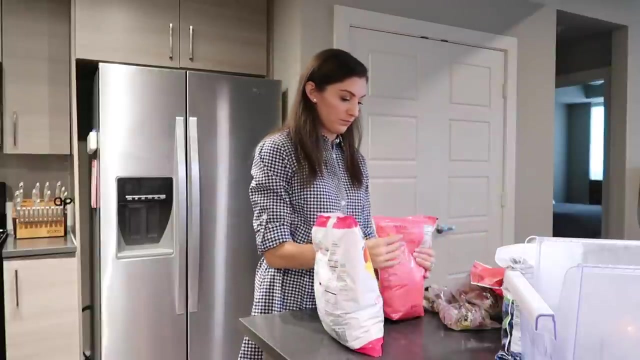 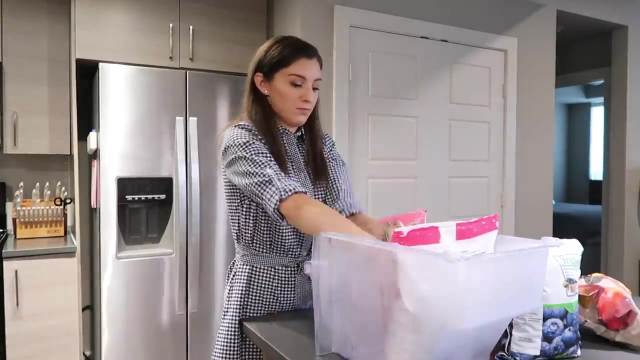 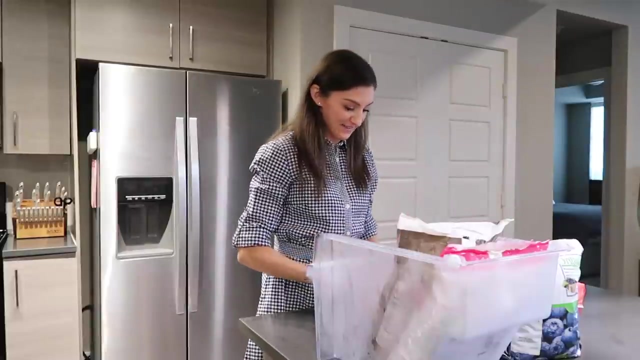 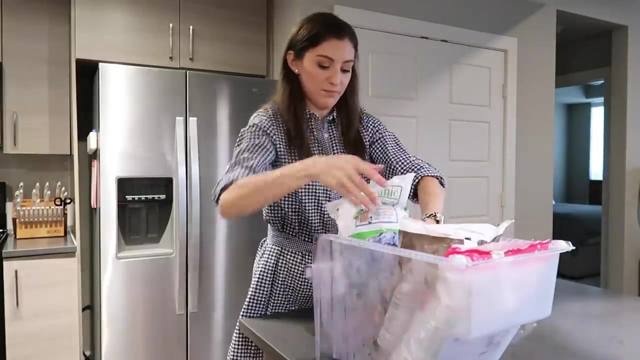 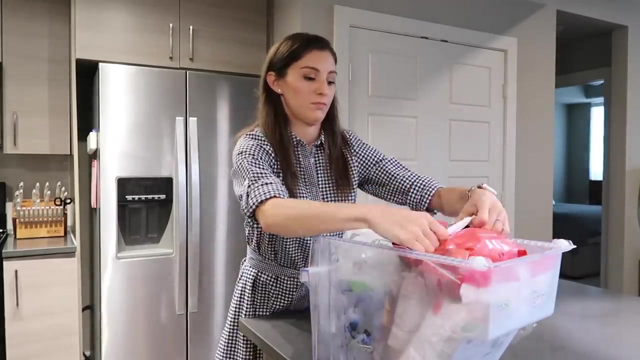 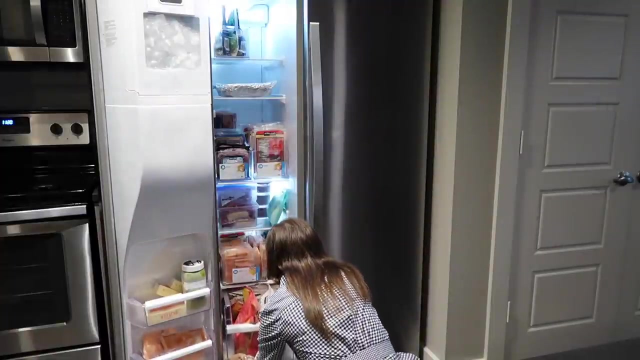 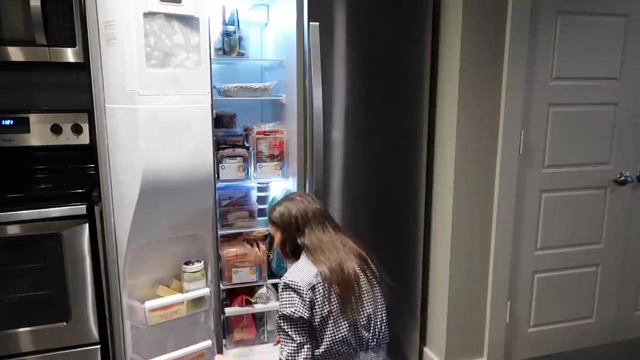 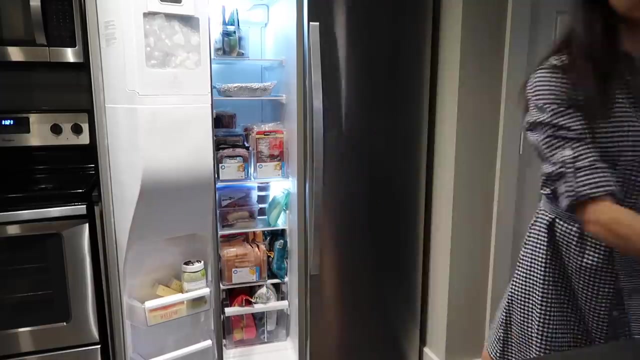 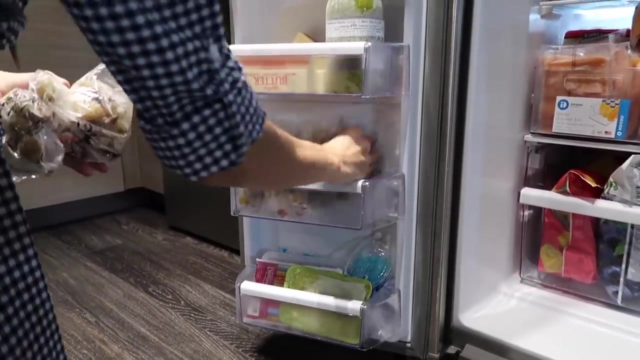 Don't mind me, while I sneak a blueberry that I spilled, Go ahead and cut the rest into two equal parts and put them into a blender. so, last but definitely not least, is the door of the freezer, and here i just have some butter, that pesto that i really like from costco, and then i have some individual packs of frozen grapes. 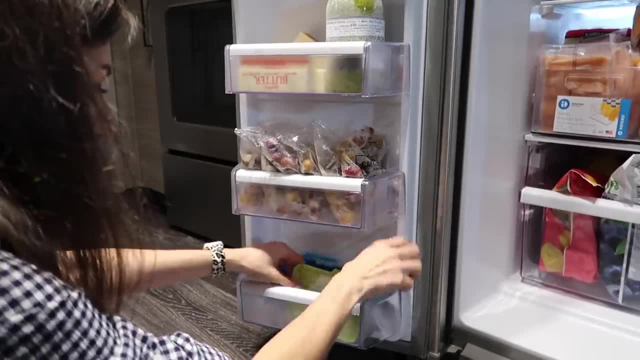 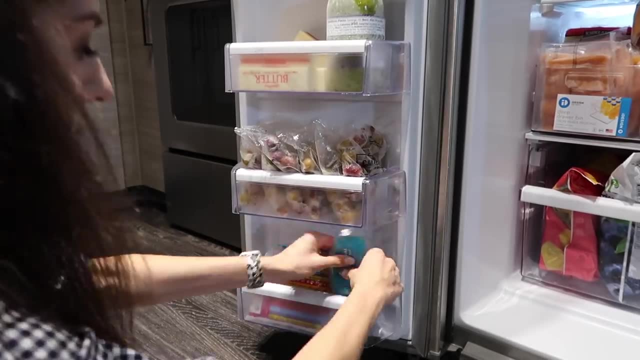 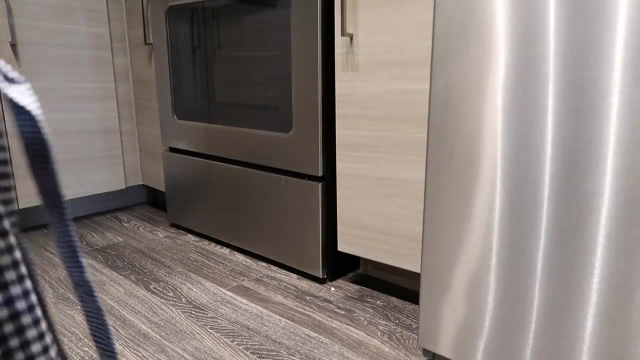 honestly kind of an impulse buy. i probably won't buy them again, so once they're eaten up, this spot will probably be empty, and at the bottom i have all of my ice packs. labels are always the finishing touch and i always get questions about where i get my labels from, and 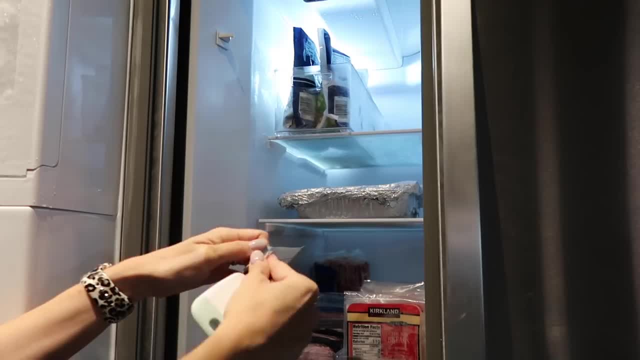 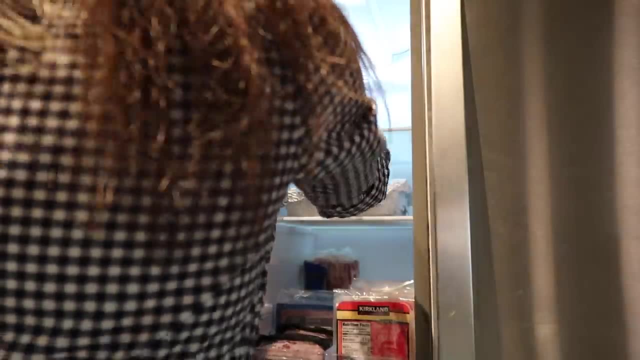 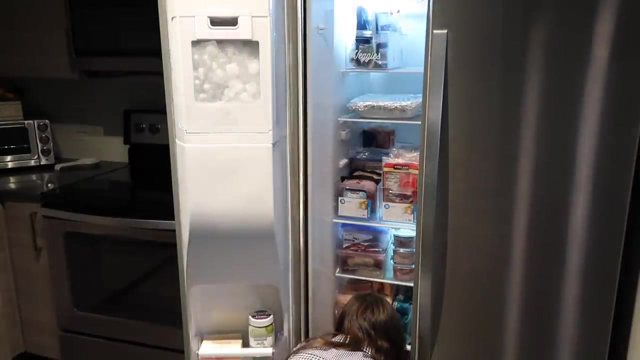 i actually make them myself. so if you ever are interested in a custom label set, just make sure to reach out to me at sophisticatedorganization at gmailcom, and we can always talk about a custom label set for you. but i think the labels totally pulled this freezer together. it did look organized. 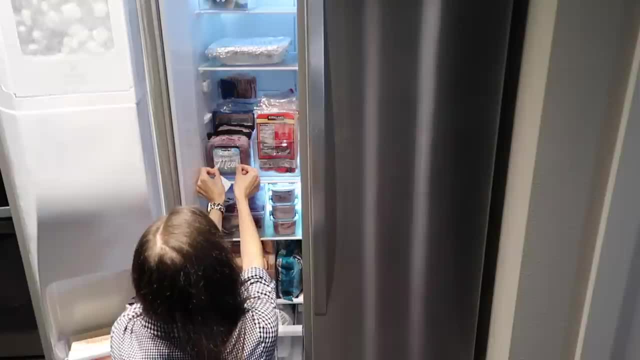 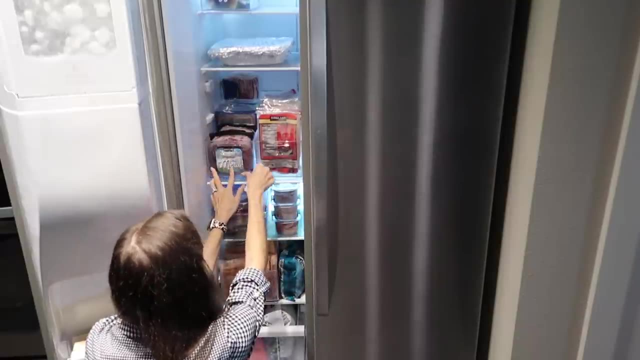 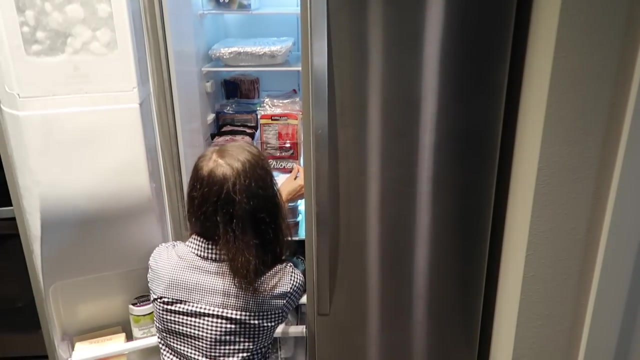 with the bins, but the second. i put those labels back on and stepped back and looked at everything. i'm in love with it. why don't we talk about this? why don't you stay, stay. why don't we talk about so, if you guys have been following me on instagram or on youtube for a while? 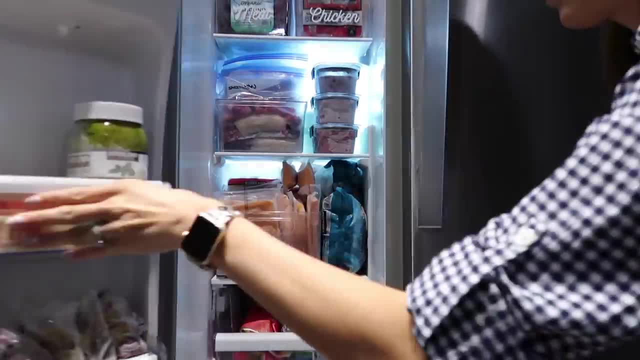 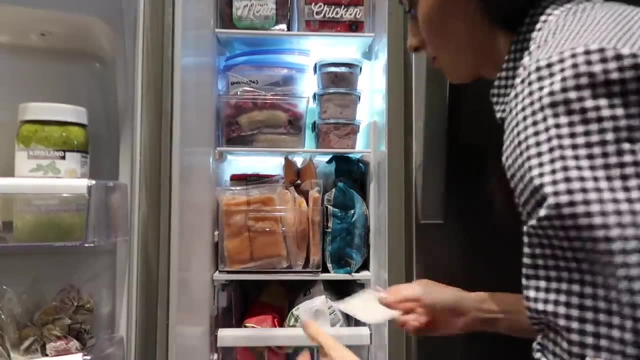 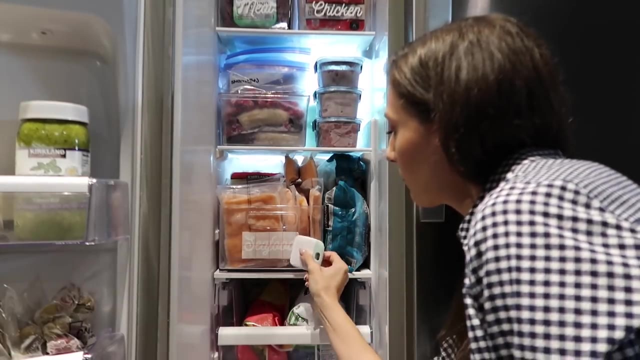 you know that i like using the freezer as much as possible, especially for meal prepping, and you'll see, i only have one freezer meal left right now, and it's in that tinfoil casserole dish and that spot. i can easily stack one or maybe even two more dishes on top of it, but i also have room. 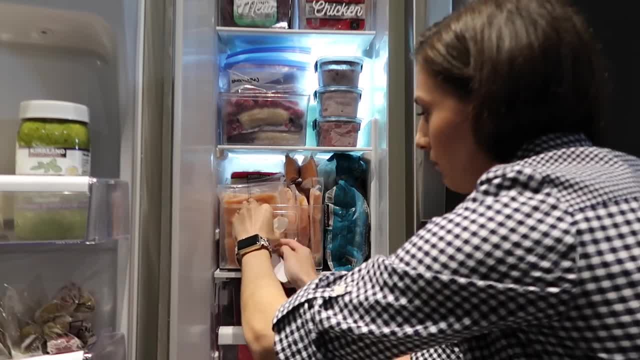 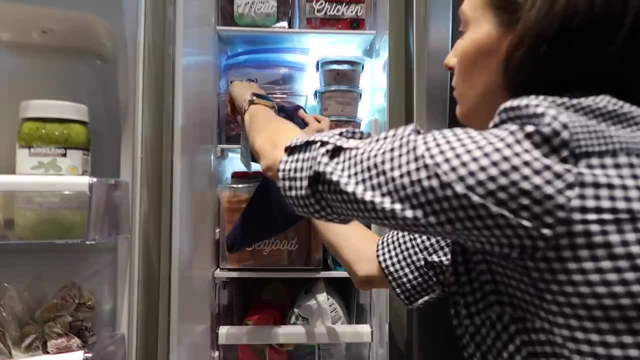 right next to my veggie container for other smaller frozen vegetables, and i'm going to put some more frozen meals or any little items i might need to stick in there. so this freezer does definitely leave a little bit of space for me to put some more items in there. 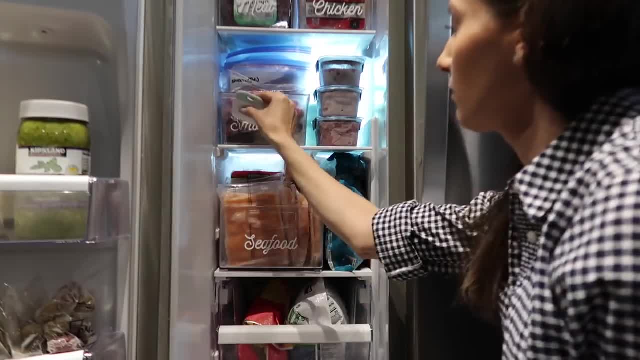 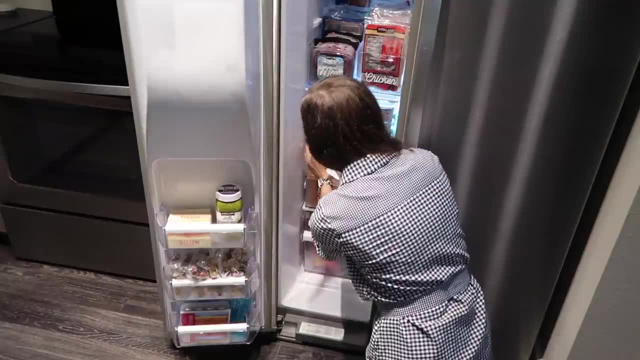 but guess i need more of you with us. it's all or nothing, but guess i need more of you. say you're doing night, but i'm wanting you to sleep with us. it's all or nothing. you and me stuck on the ocean now. nothing but the ocean now. 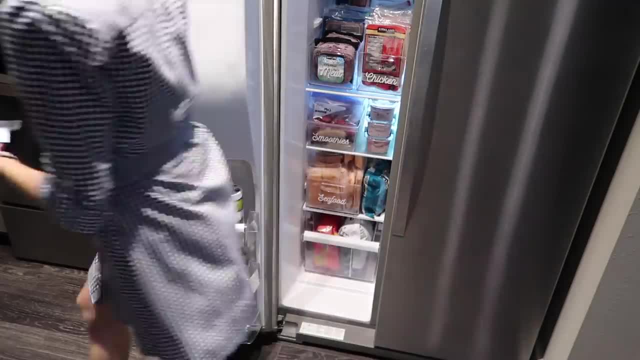 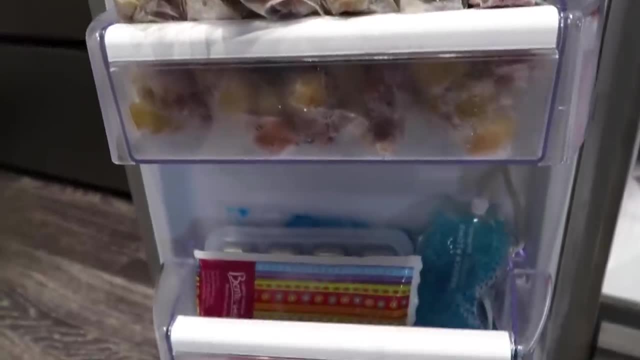 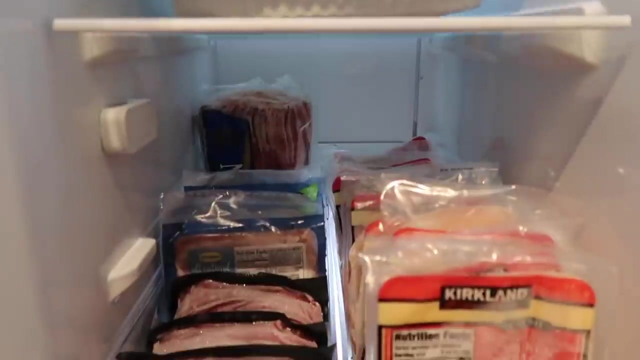 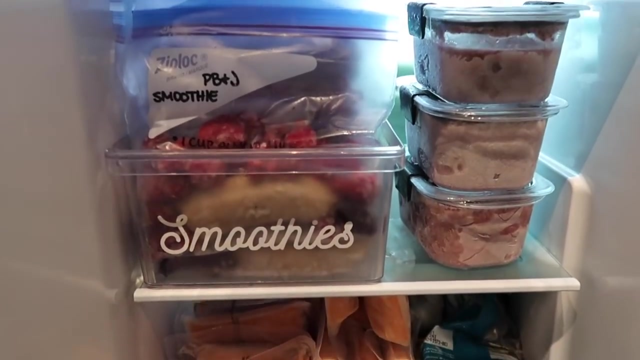 nothing, but the ocean now waves and they're spilling in. i want to dry up a chew. just keep on going, don't you? i don't even know how we got here. all my reasoning have disappeared. i want to bury the hatchet and find the way back to our home, our home, our home. we don't have to drift inside this dome. 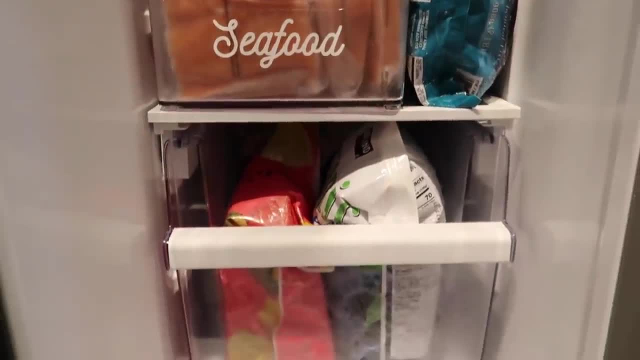 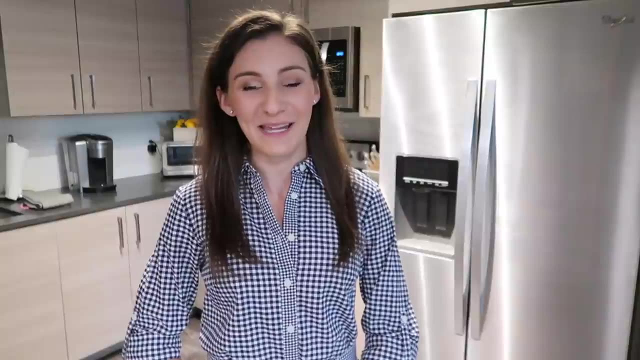 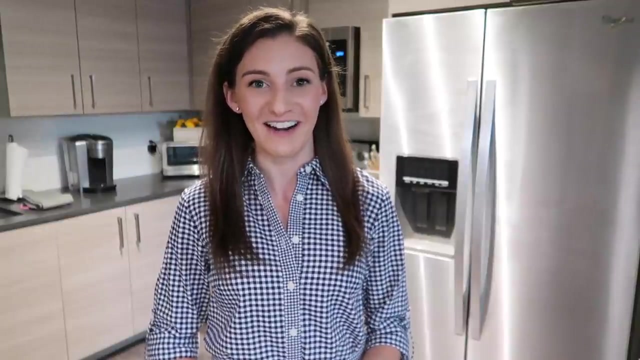 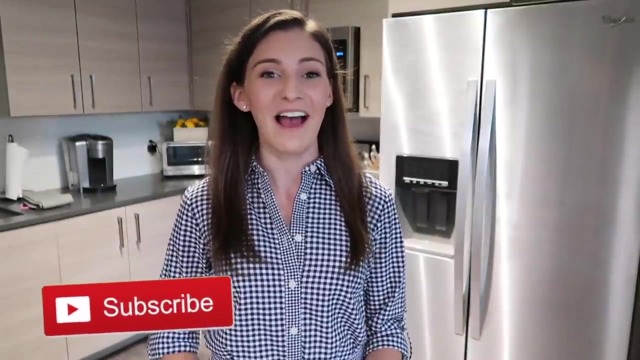 i will not. let us fade away, it's not a problem. okay, everyone, the freezer is officially organized. it only took a couple of bins, some labels and then coming up with different categories and a place for each type of food in the freezer. so if you guys like this video, make sure to give the thumbs up, subscribe to my channel for more. hit that notification bell. i have plenty more spaces to organize in my new apartment. so stay tuned and until next time i will see you guys later. you. 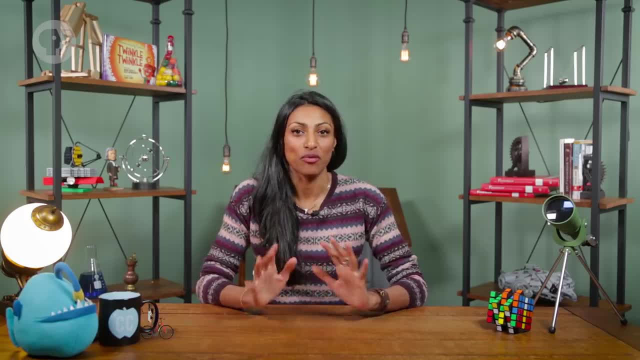 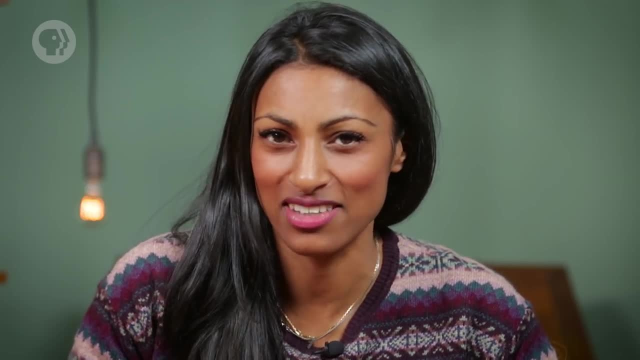 So far, we've spent a lot of time predicting movement – where things are, where they're going and how quickly they're going to get there. But there's something missing, and something that has a lot to do with Harry Styles And 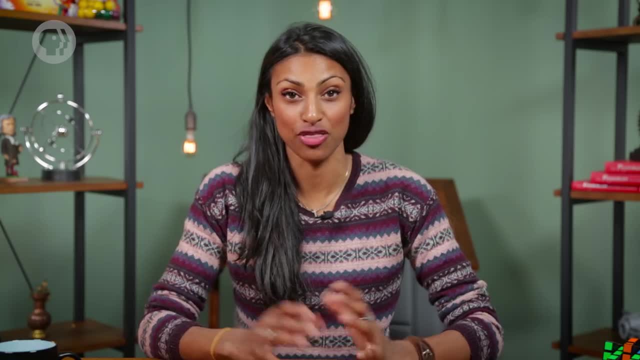 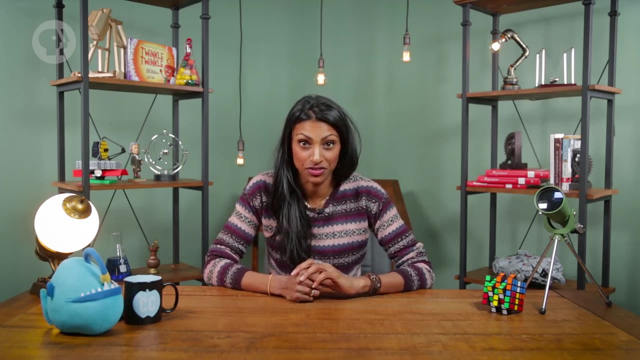 today we're going to address that. We've been talking about what happens when you do things like throw balls up in the air or drive a car down a straight road. That kind of motion is pretty simple because there's only one axis involved: The car's. accelerating either forward or backward. the ball's moving up or down. there's no messy second dimension to contend with, But this is physics. We may simplify calculations a lot of the time, but we still want to describe the real world as best we can And in real life, when you need more than one direction. 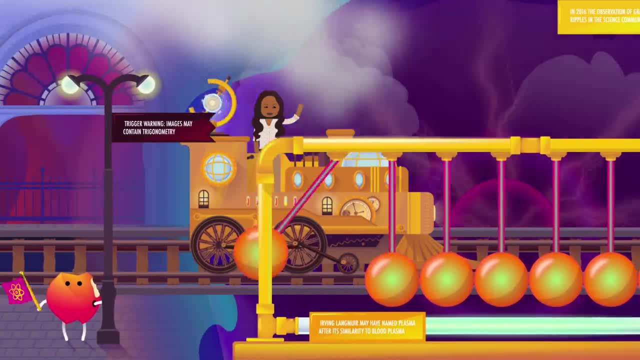 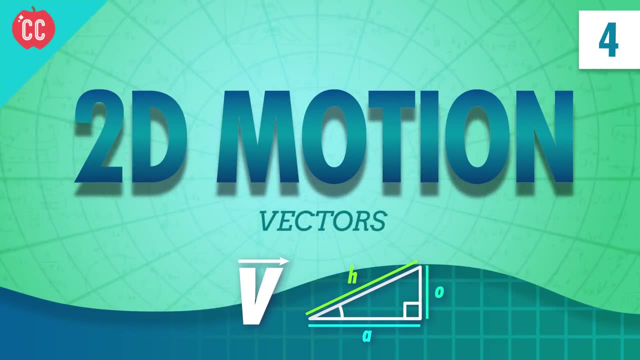 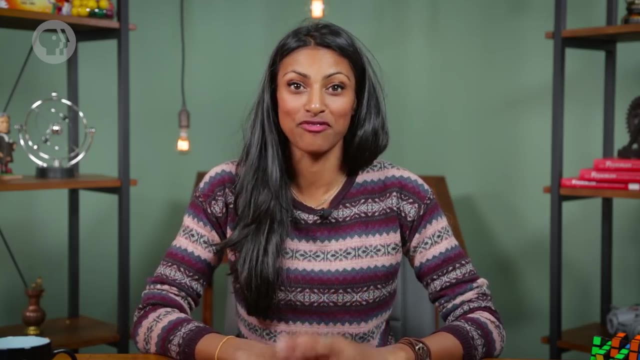 you turn to vectors. Let's say we have a pitching machine like you'd use for baseball practice. We're going to use it a lot in this episode, so we might as well get familiar with how it works. We can feed the machine a bunch of baseballs. 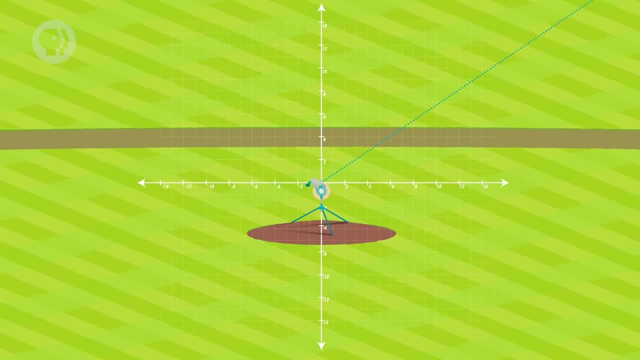 We can feed the machine a bunch of baseballs. We can feed the machine a bunch of baseballs balls and have it spit them out at any speed we want, up to 50 meters per second. The pitching height is adjustable and we can rotate it vertically so the ball can be launched. 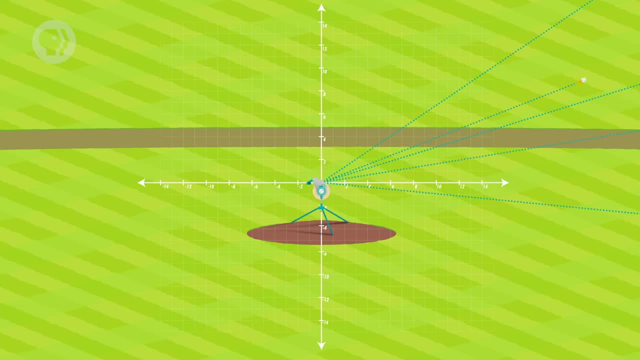 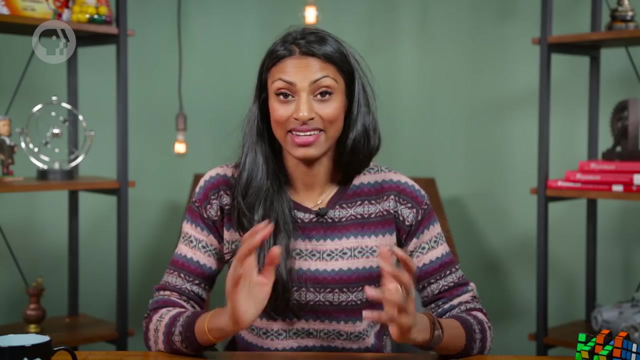 at any angle. It also has a random setting where the machine picks the speed, height or angle of the ball all on its own. Suddenly, we have way more options than just throwing a ball straight up in the air, And now the ball can have both horizontal and vertical qualities at the same time.